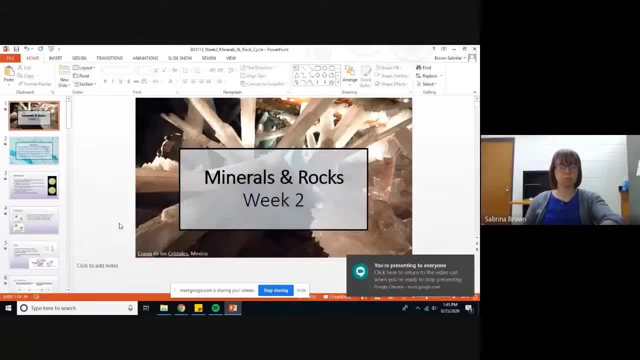 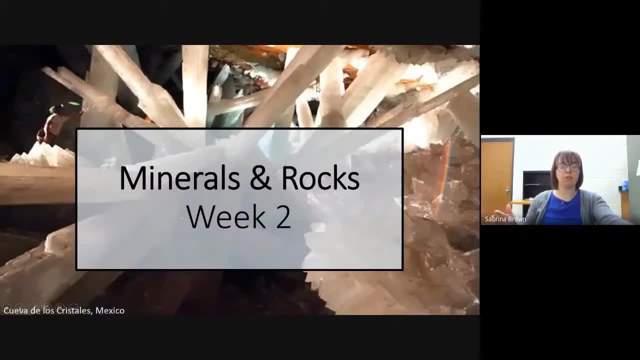 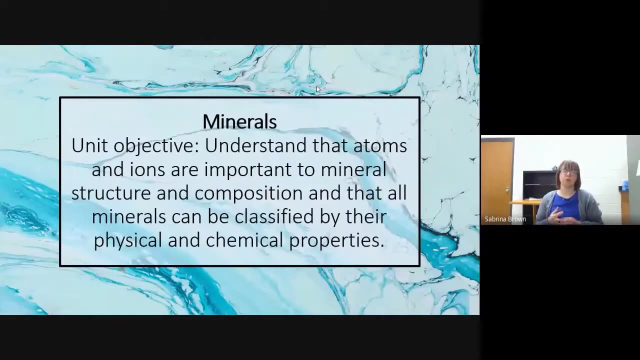 Hey guys, so today we are going to have a lecture over minerals and rocks, And so really, we just want to understand that atoms and ions are important to mineral structure and composition, And we want to understand that all minerals can be classified by both their 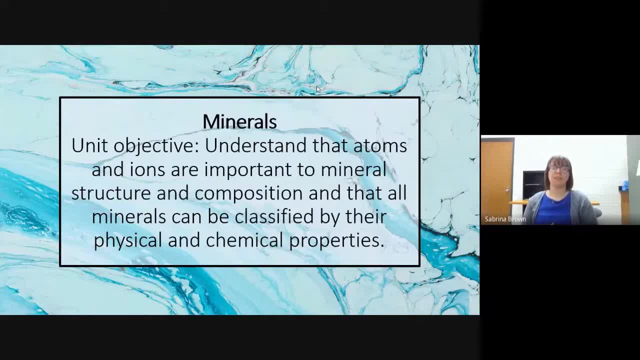 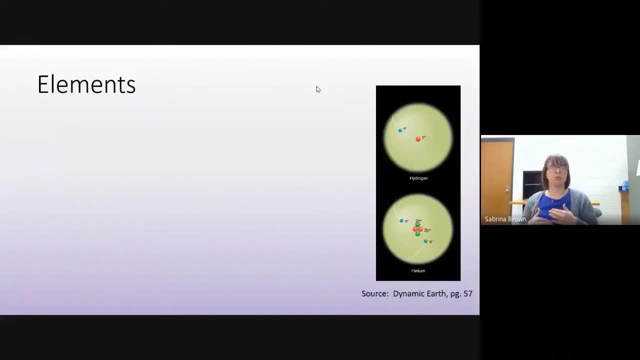 physical and chemical properties, And then we will talk a bit about rocks and how rocks are composed of minerals and that there are three different types of rocks. So before we start thinking about minerals, we have to first think about elements, And that's because minerals are the building blocks of rocks, So rocks are made up of different minerals. 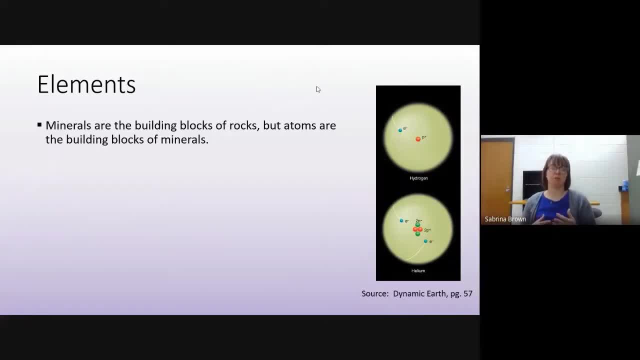 But atoms are the building blocks of minerals. So before we talk about minerals we have to talk about elements and atoms. So sort of going back to chemistry class. And so remember that an atom is the smallest unit of an element that still possesses the properties of that element. So 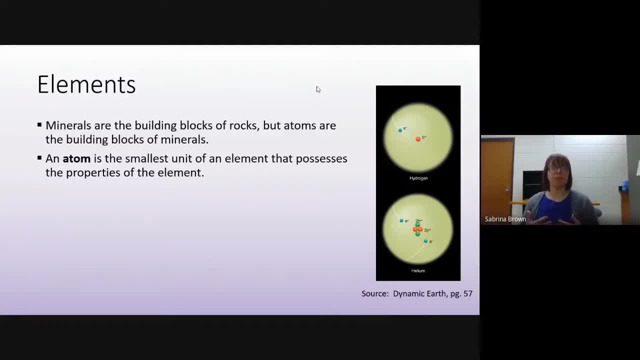 if we're thinking about different elements like hydrogen or helium. an atom is that smallest piece that still has the properties of hydrogen or helium. And remember that an atom has a nucleus made up of protons and neutrons and is surrounded by a cloud of electrons, And protons are positively. 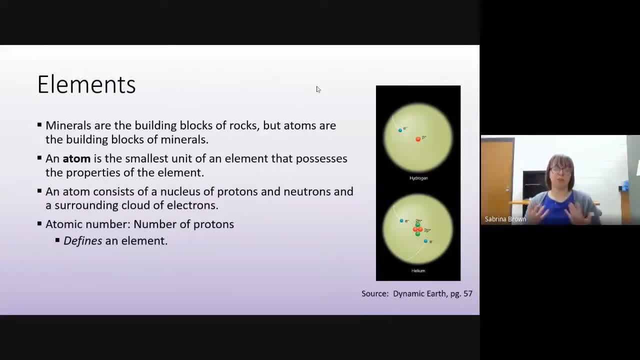 charged neutrons are neutral and electrons are negatively charged. And so remember, on the periodic economy class, with the atomic numbers of protons, We're looking at 2 protons and neutrons and they could be written as 0. But then if we wrote 1, same number of protons, 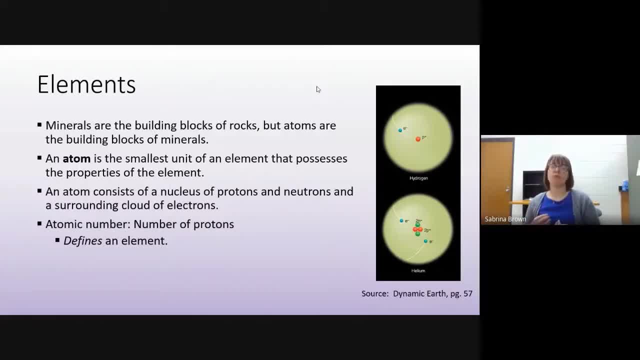 it would be the same: a number of protons That can be balanced in three different ways. So 1 protons is the number of protons that an atom has, And that's what defines the element Right. so hydrogen has one proton, So it has an atomic number of one. Helium has two protons, so it has an atomic number of two. You can see that over here How we have 1 proton in hydrogen and we have 2 red ones, 2 protons in helium那 mosque喔 Thì có nh cin và Нетudaее thей cóCu document. wish ol öy th cuánt v scan problema á cholesterol. y forecast expires. 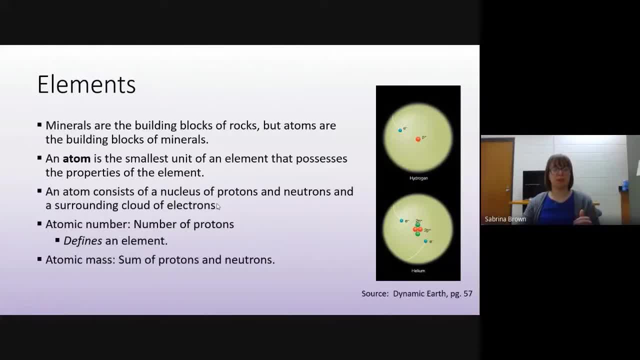 n музыч가지h modeí trong bi éo đồng mới còn لتُm. mass is basically the nucleus, the sum of the number of protons and neutrons. So hydrogen has an atomic mass of one because it has no neutrons and one proton. 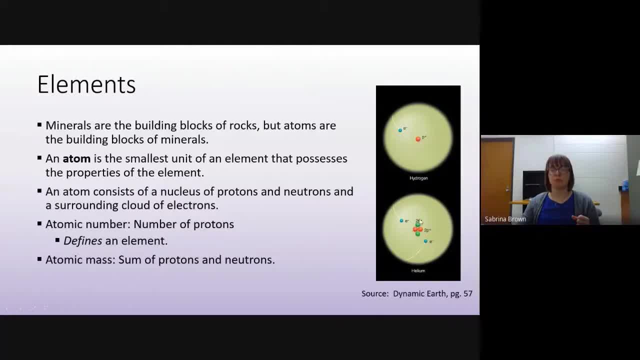 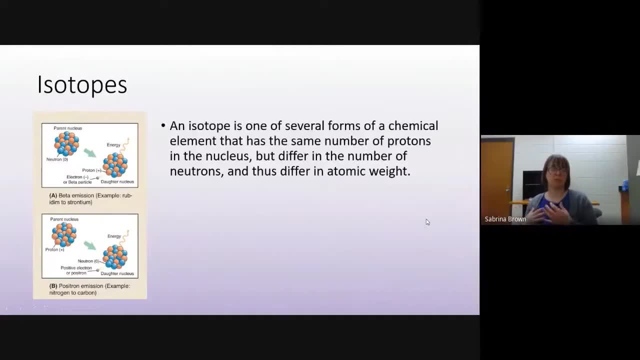 Helium has an atomic mass of four because it has two protons and two neutrons. All right, so we have atoms. We reviewed atoms a bit. Now let's think about isotopes. So remember that isotopes are just different forms of an element that have the same number. 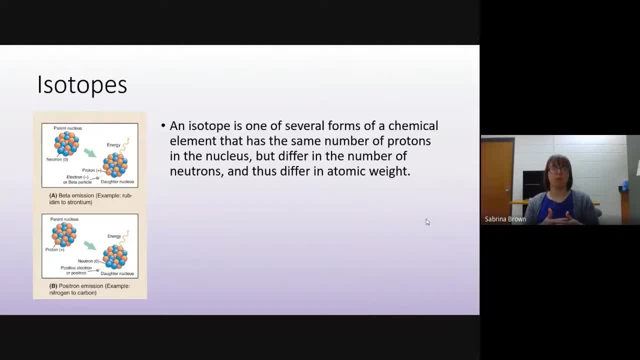 of protons but a different number of neutrons. And so since there's a different number of neutrons, there is a different atomic weight. So most elements, most atoms of an element, have a certain number of protons and a certain number of neutrons. But if you have a different amount, 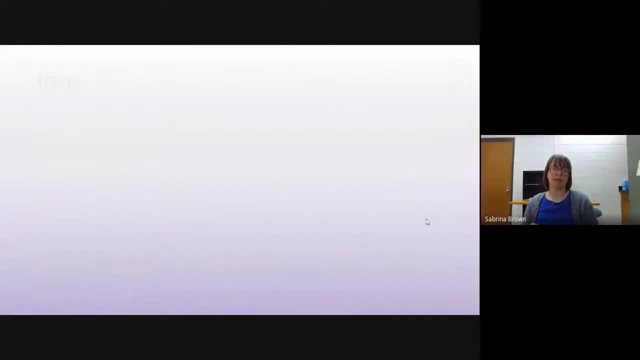 of neutrons from sort of that base, you have a different number of neutrons. So if you have a different number of neutrons from sort of that base, then we call that an isotope And then remember that ions are when we have more or less neutrons than sort of a regular. 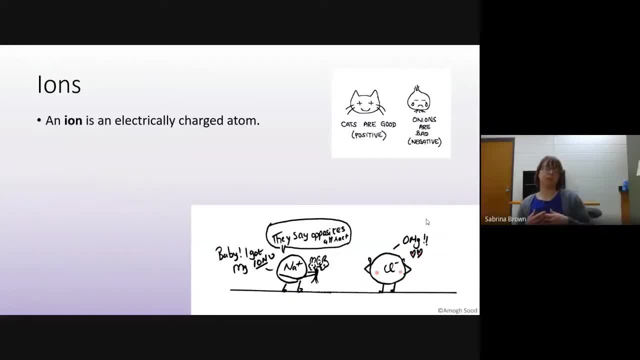 atom of that element would have. So that's why we call ions electrically charged atoms. And so when you lose an electron- since electrons are negatively charged- if you lose one that makes your ion positively charged, We call that a cation, and i always learned to remember cation. the t is like a little positive. 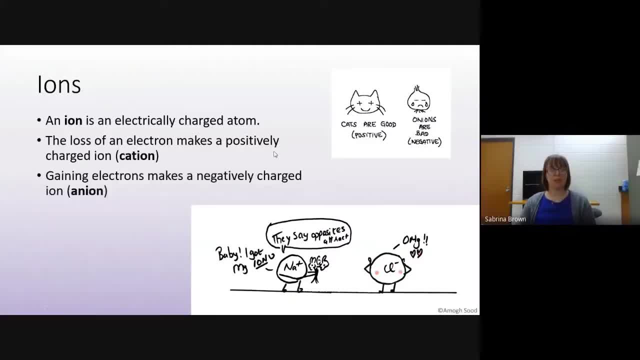 sign. so cations are positive, and then anions are, when you gain electrons and thus have a negatively charged ion or a negative ion- And remember that ions, because they're electrically charged, a positive and a negative useま negative ion- are going to attract each other, And so I just wanted you to have a couple of those. 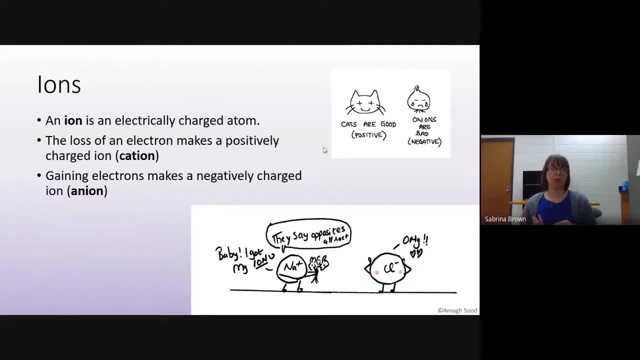 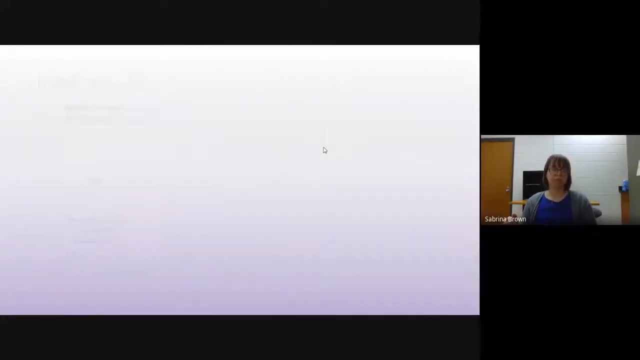 sort of chemistry definitions, of remembering what elements and atoms are, remembering what isotopes are and remembering what ions are, because they're important when we're talking about minerals and they become important when we're talking about water and other things, the atmosphere as we move throughout the semester. So just a refresher on those guys. So when we're 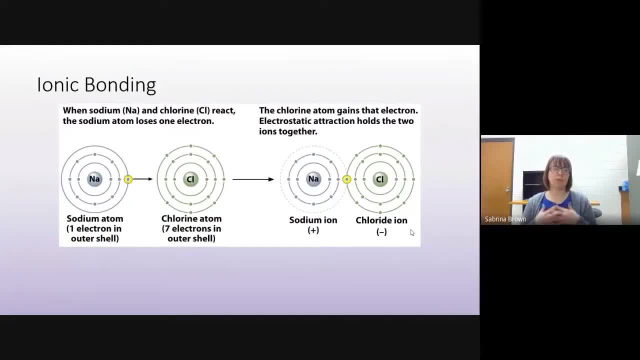 talking about minerals. we care about ions because we care about the ionic bonding process, And so there's two different types of bonds. So when we're talking about ionic bonds, that's when you have charged a positive and a negative ion that are attracted to one another. So in the diagram, 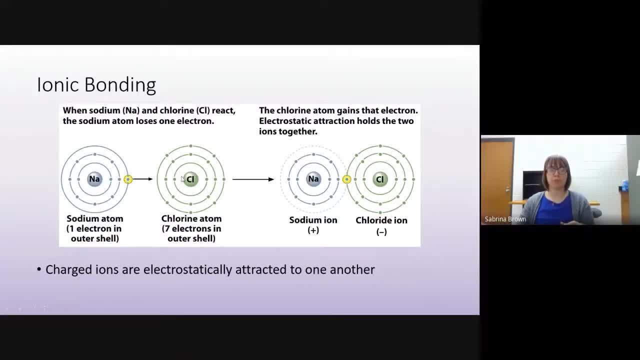 we have positively charged ion and negatively charged ion, And then we have positively charged ion and negatively charged ion, And then we have positively charged ion and negatively charged ion, And then we have positively charged ion and negatively charged sodium, negatively charged chloride, and they are attracted to each other, And so they have sort of this: 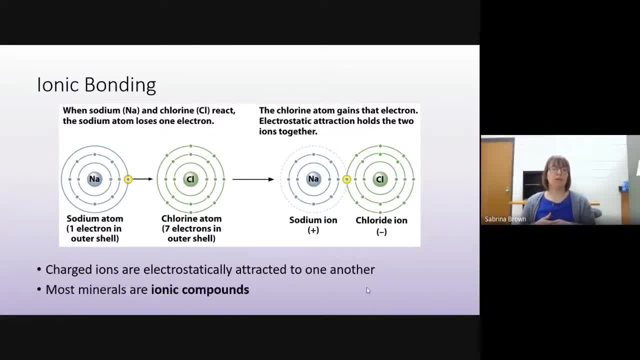 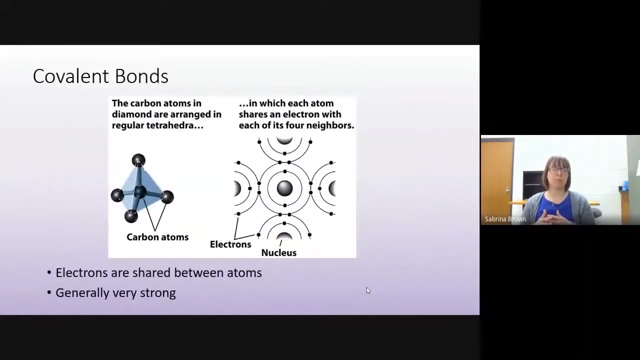 weak attraction to each other that holds them together. And most minerals are ionic compounds, right, So we care about ionic bonding, because most minerals are made up of ions, negative and positively charged atoms stuck together by those charges, And there's also covalent bonding, which happens usually in carbon atoms. So that's why diamonds are. 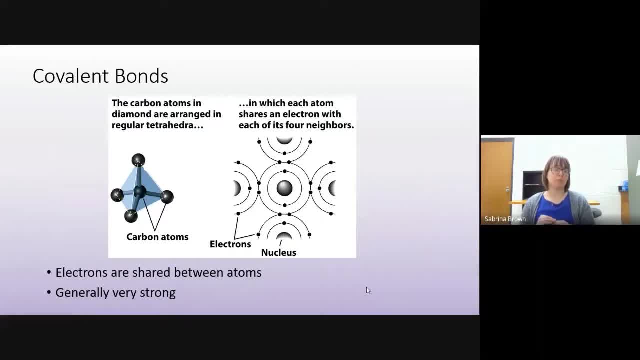 so strong because it's a bunch of carbon atoms arranged in covalent bonds, And so remember that covalent bonds are when electrons are shared between atoms, right? So the atoms are sharing them, So you have a really strong bond, instead of just being sort of attracted to each other. 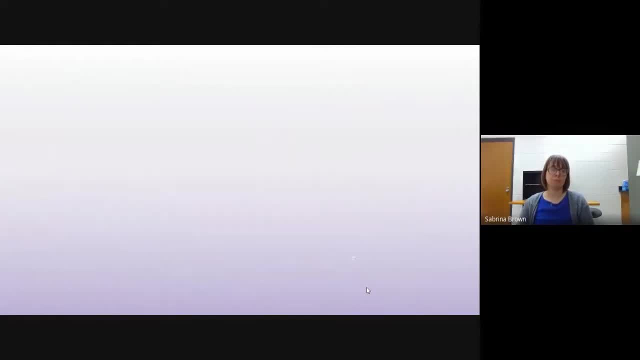 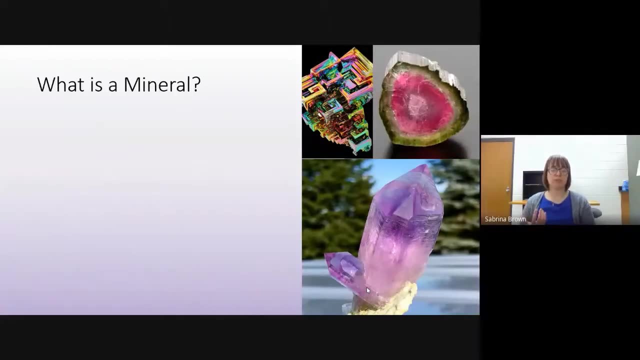 So you have a really strong bond, instead of just being sort of attracted to each other Like an ionic bonds. All right, so that was your chemistry lesson for the day. Now let's move on to the definition of a mineral. So a mineral is a naturally occurring right, So it has to be. 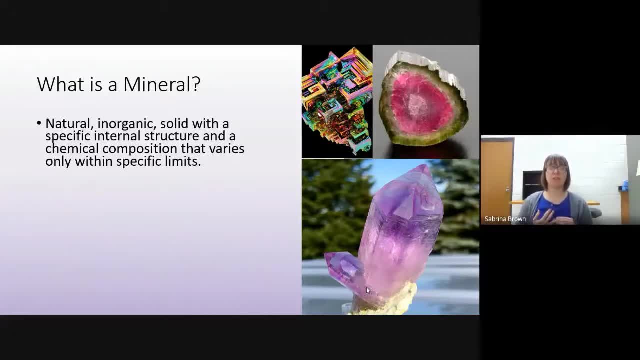 formed in nature, inorganic, solid. So inorganic means that it was not formed from living carbon, So it has to be formed from living carbon. So it has to be formed from living carbon. Solid, right. Solid at room temperature, right. Can't be a liquid, can't be a gas at room temperature. 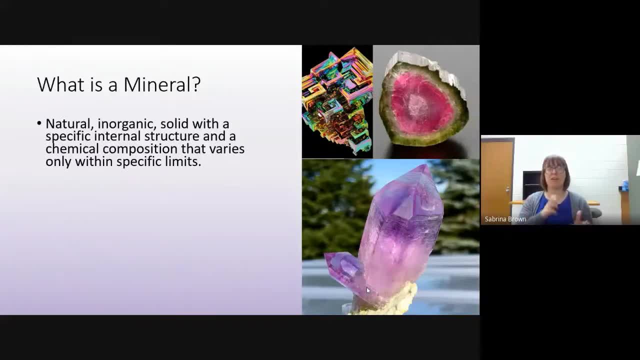 And it has some specific internal structure. So inside it has some type of ordered bond structure between the different atoms- which is why we reviewed what atoms are- And it has a chemical composition that's specific to that mineral and it only varies within certain specific limits, right? 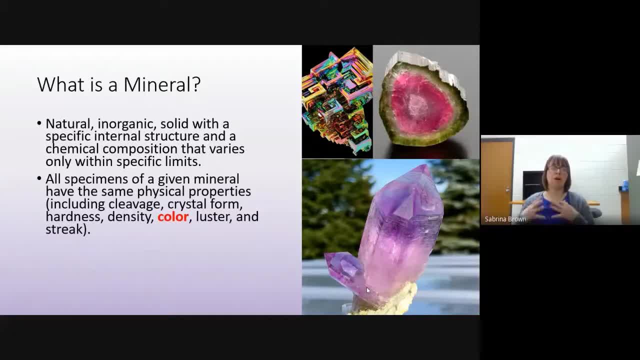 So all mineral, all specimens of a given mineral, all examples of, let's say, a mineral quartz, have the same physical properties. And so physical properties are things like cleavage, which is not what you're thinking. it is the form of the crystal: hardness, density, color, luster. 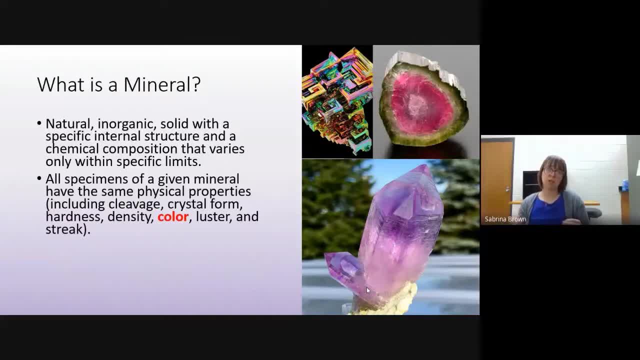 and streak, And so we'll talk about those physical properties in this lecture. but we define a certain mineral based on those physical properties, And minerals also have restricted stability ranges, which means if we heat them up a little too much or we subject them to too, 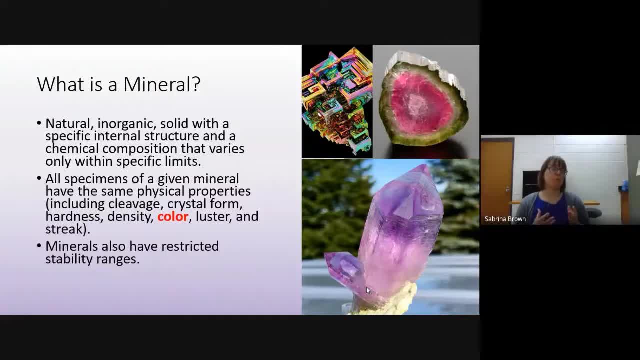 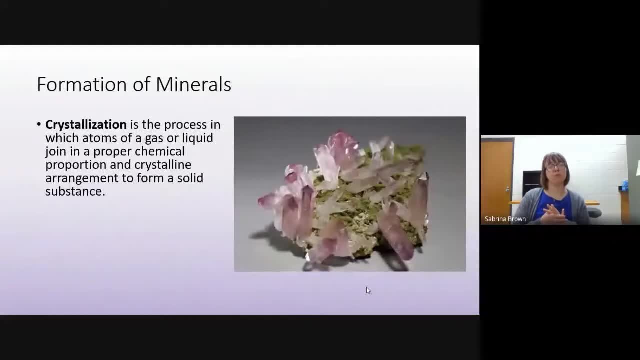 much pressure, they are no longer going to remain that mineral and they will change in some way. Okay, so minerals form through the process of crystallization, And crystallization is just the process where atoms, either in a gas or a liquid, come together and form a solid right. 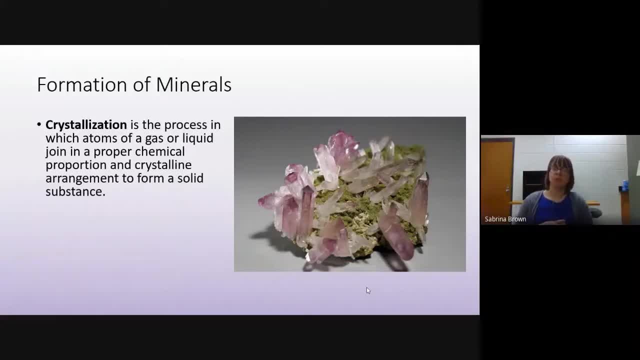 So think about in chemistry class when you put a liquid and a liquid together and then all of a sudden something precipitates out as a solid. That's how minerals form. through this process. Minerals form through the process of bonds being created between different elements. 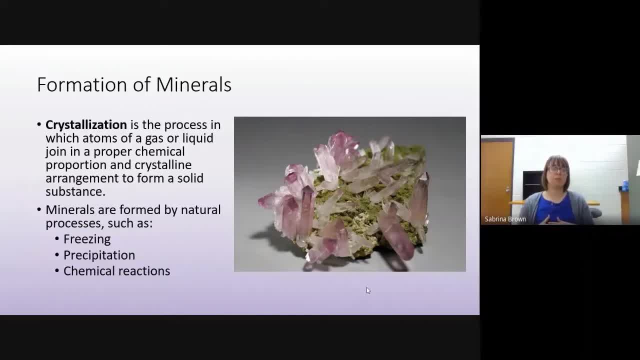 And that crystallization process, forming this solid substance in nature, happens through freezing right. So you can turn liquid water into a solid by freezing it. Minerals are formed in similar processes. through cooling down. they can form through that process of precipitation where different ions in the water 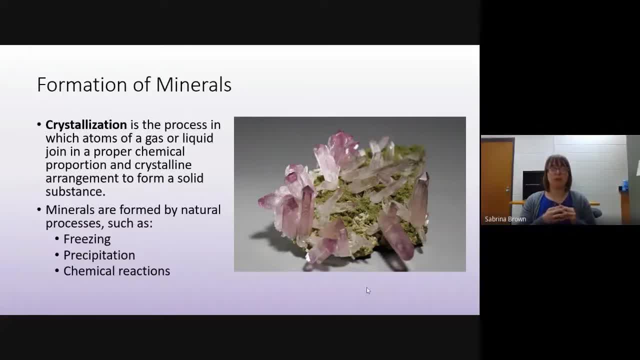 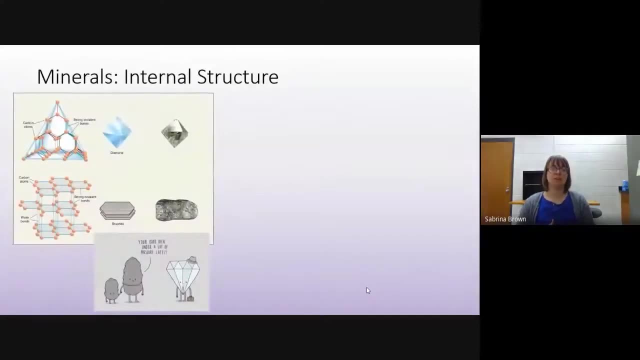 come together in the right proportion that they turn into a solid, and also through a number of other chemical reactions where this chemical is reacting with this one, and then you have some product that is a solid Again. thinking back to your stoichiometry in chemistry, if you were ever. 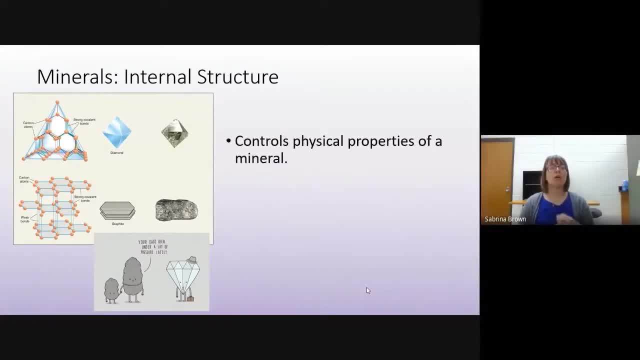 into chemistry, And so minerals have a specific internal structure, and that specific internal structure- that's just how the atoms inside the mineral are arranged and related to one another- is what actually controls the physical properties of the mineral. For example, diamonds- So think of diamonds in- diamond rings, right. 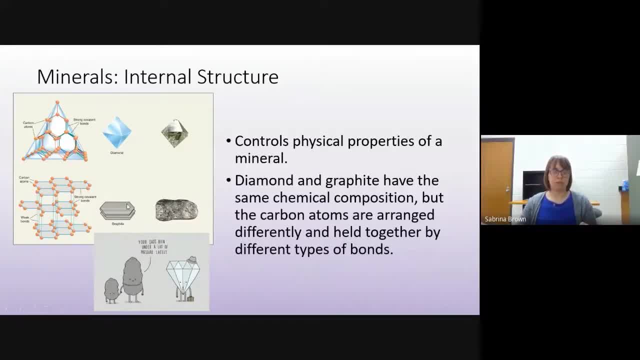 and graphite, which graphite is found in pencil lead? those have the same chemical composition. They're both made up of carbon atoms, but those carbon atoms are arranged differently within the internal structure of the mineral and they're held together by different types of bonds, right? 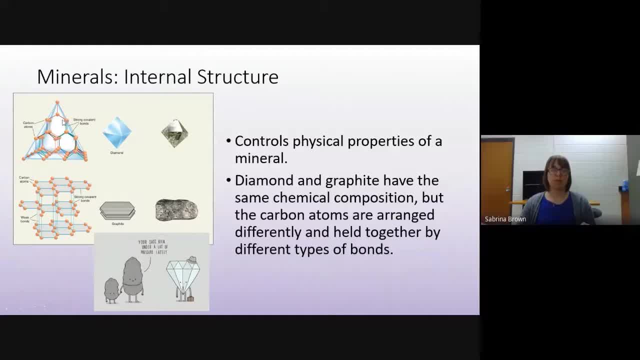 So in our diamond the carbon atoms have really strong covalent bonds. They have this tetrahedral structure that makes those carbon bonds so strong that diamond is the hardest mineral on the scale we use for mineral hardness. And then with graphite, still we have carbon atoms, still we 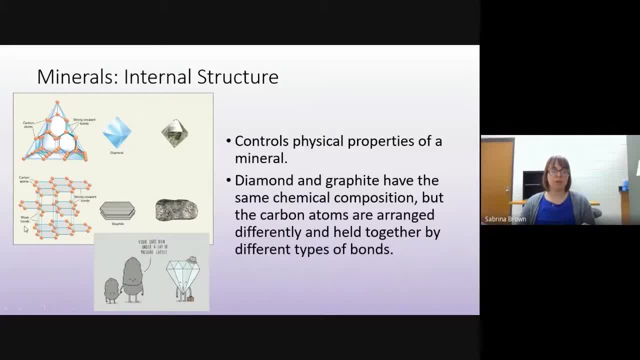 have covalent bonds, but we also have weak bonds, And so what we get with the carbon arranged in graphite is we get these sheet sheety layers that slide past each other, And then that breaks easily- easily enough that you can write on paper with graphite. 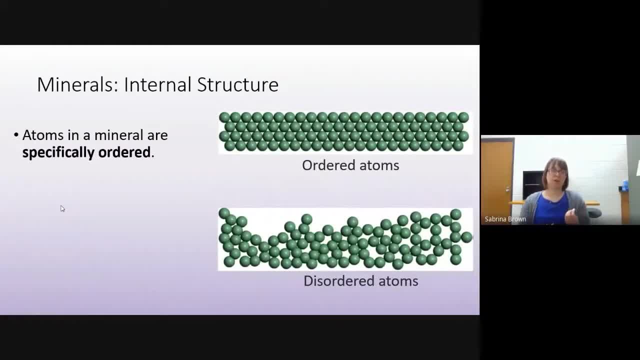 All right. so the atoms within a mineral are specifically ordered, And what that means is that they have a specific structure, And so that means that they had enough time to cool, that they were able to arrange in a bonded structure. Not all things have a specific internal structure, And if you have a solid that has a disordered 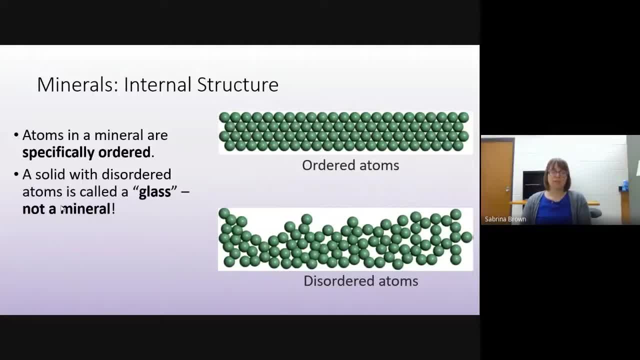 internal structure that is called a glass, And so, for example, this is how we form the glass that you think of when you think of window panes. We also naturally form glass using lava right, So volcanoes form glass, something called obsidian. 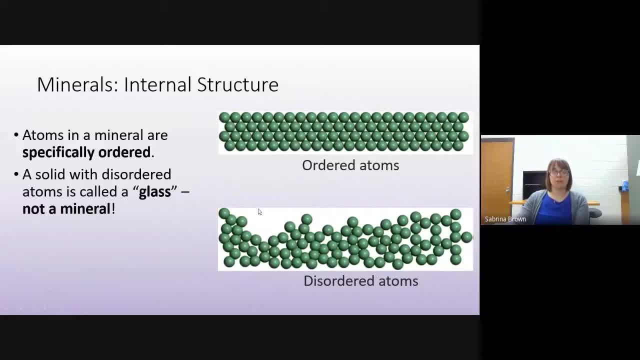 You've heard of obsidian before and we'll look at some obsidian in class. when we look at rocks, That has a disordered atom structure And so if something has a disordered internal structure, it is not a mineral, It's a glass. Minerals have to have this structure where there are bonds that 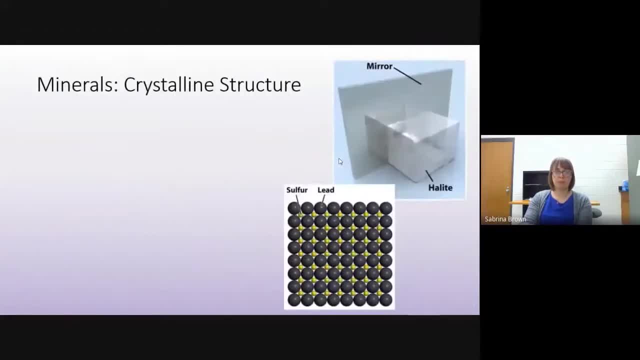 are ordered in a specific way, all different ways that you can order atoms within a mineral, but they form some type of pattern, So those bonds repeat in a three-dimensional way and so if you get on this website here you can kind of click around and look at. 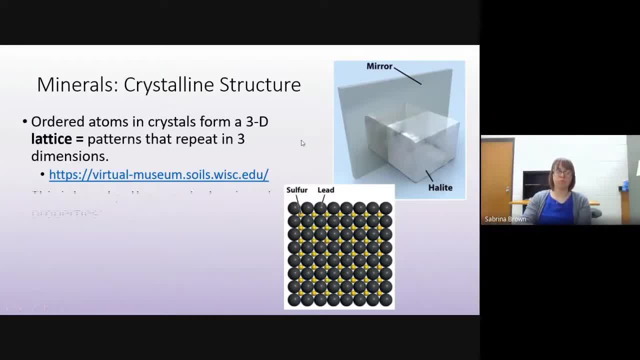 different 3D models of mineral crystalline structure. The important thing to know about crystalline structure is that the fact that the atoms in a mineral are internally ordered in a pattern controls the properties of the mineral, So it's going to control the shape of the crystal that forms from the mineral. 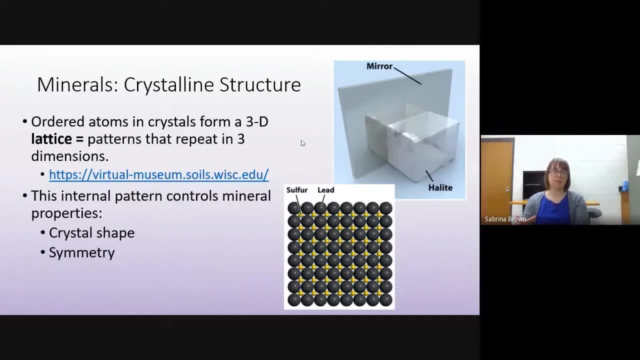 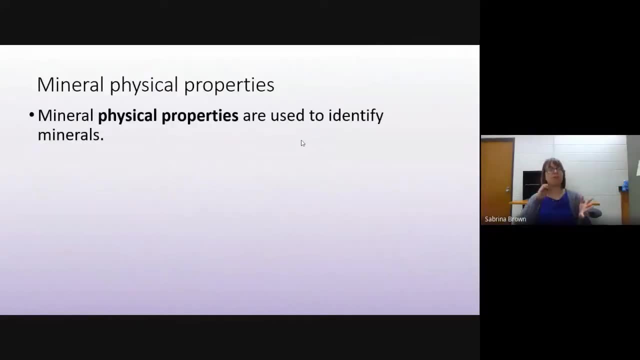 right, So what the mineral looks like is related to that internal structure, and whether or not the mineral is symmetric is um determined by this internal pattern. All right, so that's sort of the background as to why what a mineral is and why they have this internal structure. but the 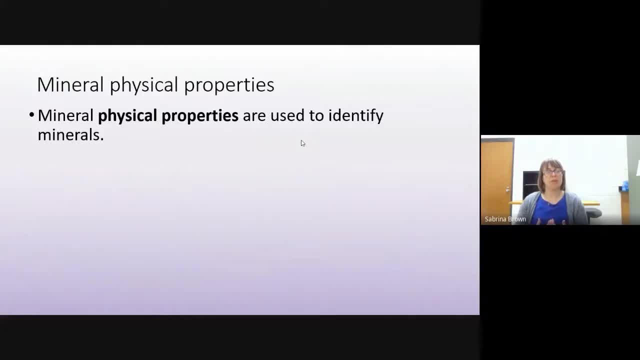 internal structure of a mineral and the elements that a mineral are made up of are reflected in the minerals physical properties, And so a minerals physical properties are what we actually use to make a mineral are reflected in the minerals physical properties, And so a minerals physical properties are what we actually use in the lab to identify what a mineral is, or which mineral we have in a rock or in a mineral sample, And so these are the things that we are really going to be focusing on a lot in the class are these physical properties, And so, again, these physical properties depend upon the chemical composition, what elements make up the mineral and that specific internal crystal structure that we are going to be going to be thinking about when we are going to be thinking about the next step of the process. So let's jump into the next slide. 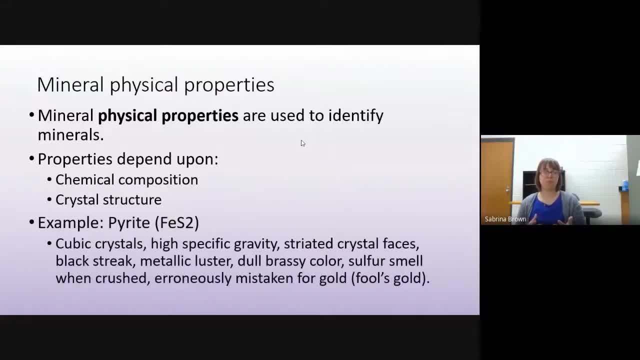 structure. so, for example, pyrite or fool's gold, we can describe it based on its physical properties. we know that it has cubic crystals, we know that it has a high specific gravity, crystal faces that are striped and when you streak it it has a black streak. it's metallic, it's brassy in color, it smells like sulfur. 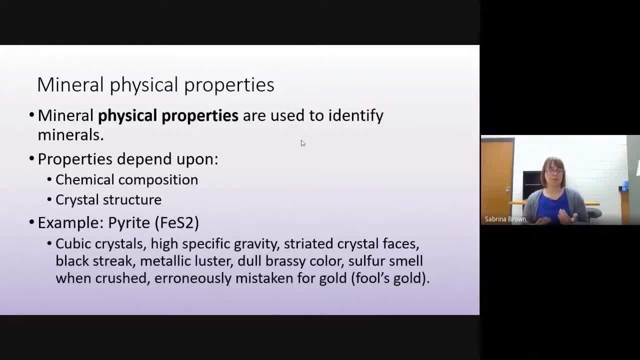 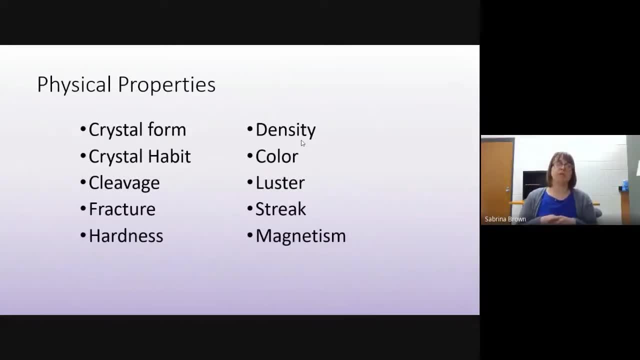 and you know, a special property is that it's often mistaken for gold. so that would be an example of using these physical properties to identify a mineral. so now we're going to go through each one of the those physical properties in turn. so there are 10 physical properties that you can use to identify. 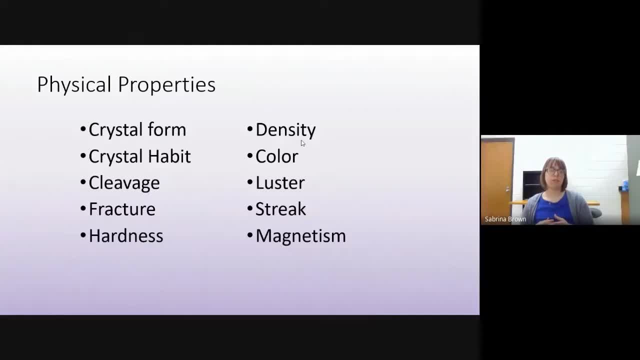 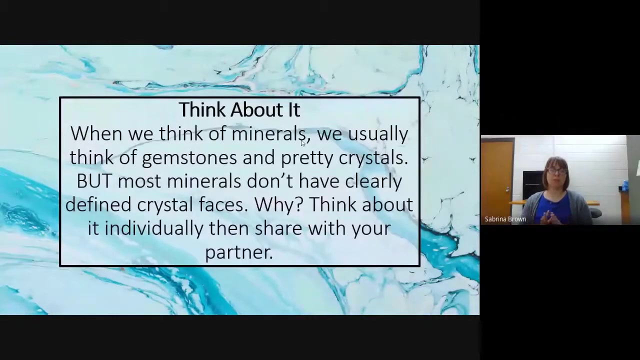 mineral in the lab or in the field so we can look at the crystal form. we'll look at crystal habits, cleavage, fracture, hardness, density, color, luster, streak and magnetism and, like i said, i'll go through each one of those in turn. so go ahead and take a minute and stop and think about when we think about minerals we usually 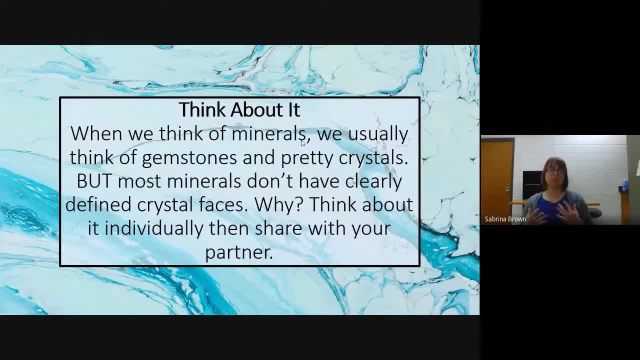 think of gemstones and really pretty crystals, right? so some people now are like into having crystals um for different healing properties, or think about diamond rings, gemstone rings, gemstone jewelry- but most minerals don't actually have clearly defined crystal faces. so think about why that is um and ignore that part where it says share with your partner, because we're doing this. 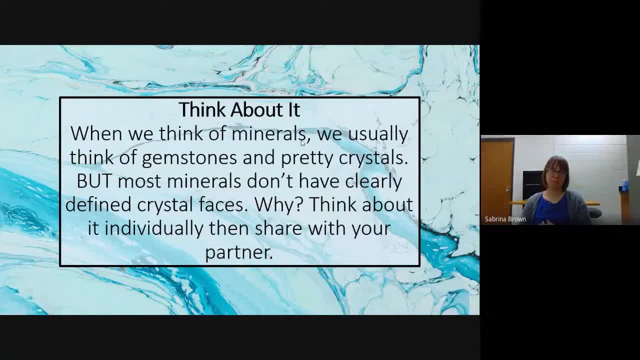 virtually this semester, and you can pause the video if you need some more time to think about that and i'll tell you the answer. okay, so crystals, naturally formed crystal faces, which are commonly what people have if they have healing crystals or they sort of collect crystals and rocks. those natural crystals are formed in nature but they have to have space to grow. 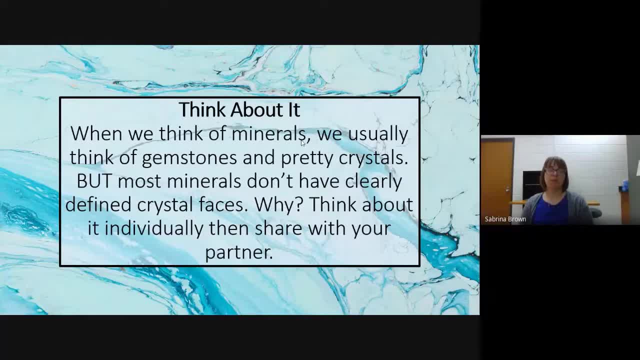 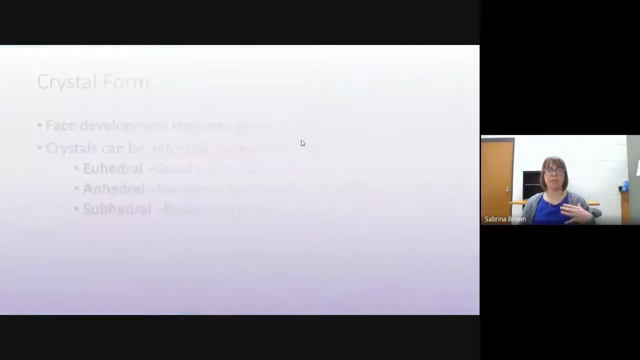 and then gemstones. usually those are a lab cut face. so they take a mineral and cut it and faucet it to make it look pretty and shiny, but it didn't necessarily grow in nature that way. so when we're thinking about naturally made crystals that have faces, this is related to something called crystal form. 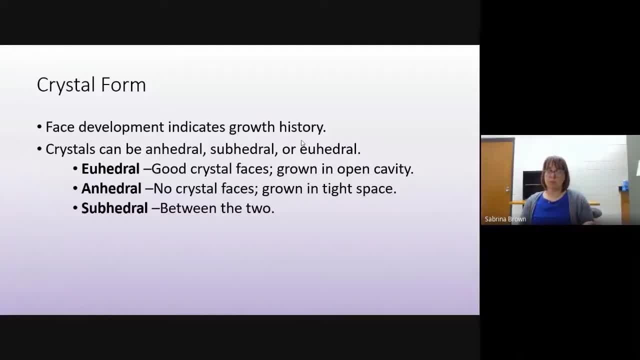 and so when you have like a really pretty crystal that formed naturally- it was a- has a eu hedral crystal form, which means that it has really good crystal faces and that had space to grow in an open cavity, um, if you have no crystal faces- which by far most- 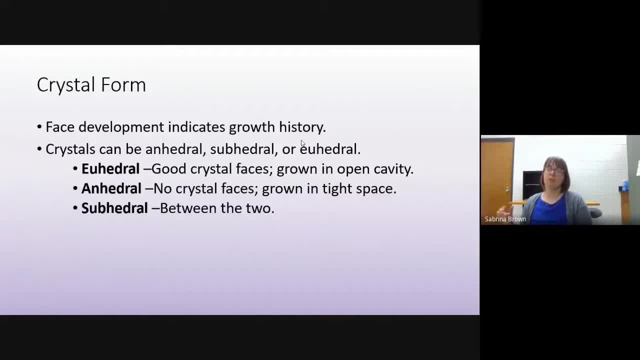 minerals have no really nice crystal faces. that means they were grown in a really tight space and again that's an hedral crystal form and then sub-hedral is somewhere between the two where it might have some good crystal faces or sort of medium quality crystal faces. 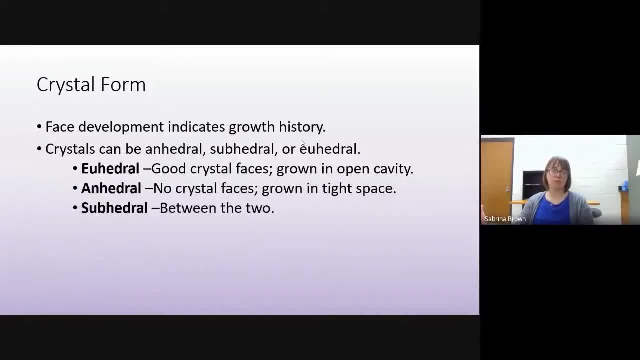 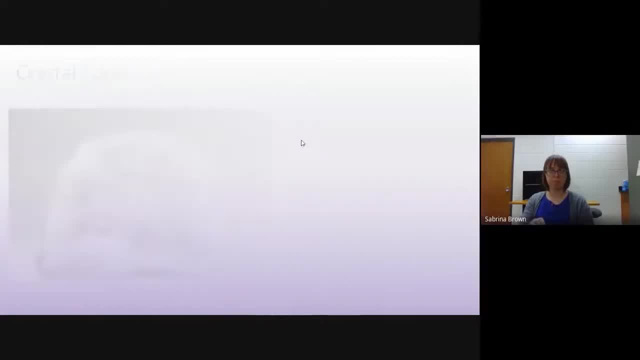 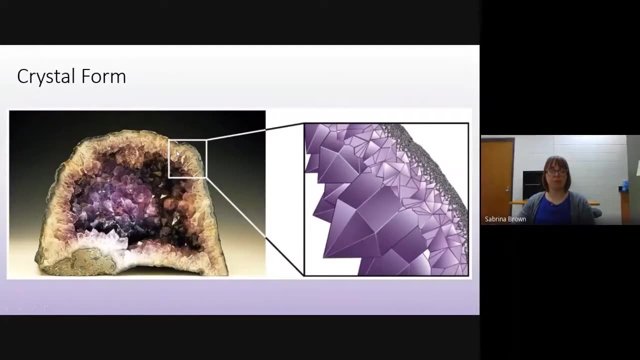 And so this form, how the crystal looks, indicates how much space that mineral had to form. So here's an example, if you think about a geode, And I'll bring one into class when we are in class next time. So we have a geode where we 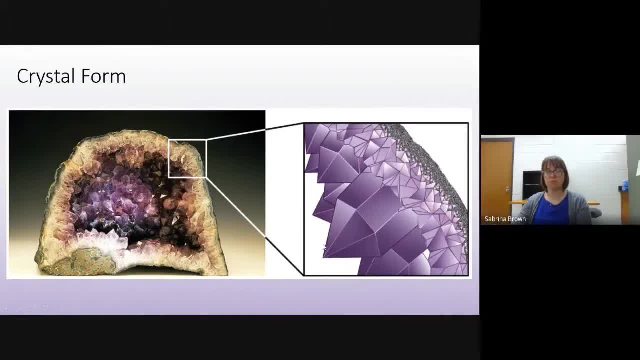 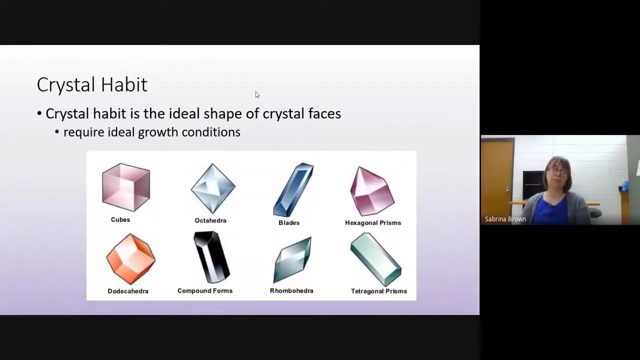 have euhedra- really pretty crystals. We have anhedra- really bad crystals here, And then in between we have some sort of sort of- okay, subhedral crystal forms in our geode here, All right. next we have crystal habit. 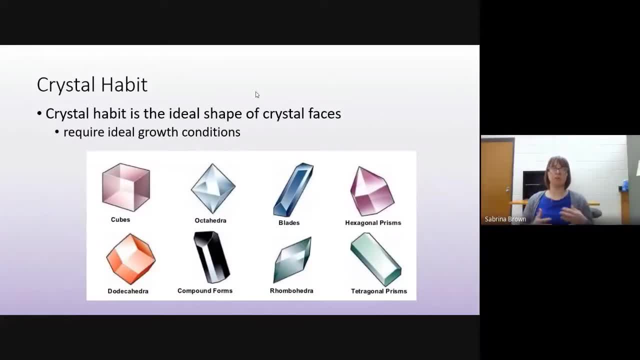 which is that if the, if the crystal or the mineral has all the space and time to grow, has really ideal growth conditions, what will the crystal faces actually look like? So crystal habit is: what form will this crystal take if it grows naturally with ideal growth conditions? 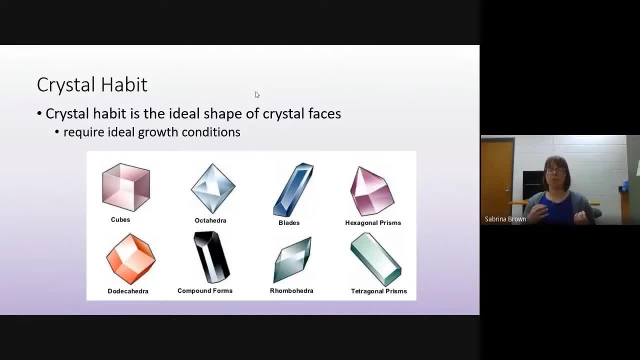 And crystal habit again is related to how those bonds and elements are bonded within in the mineral right, this internal structure. So some ones that we'll see in lab are cubes, octahedral, we'll see hexagonal prisms. I think we'll see rhombohedral. All right, 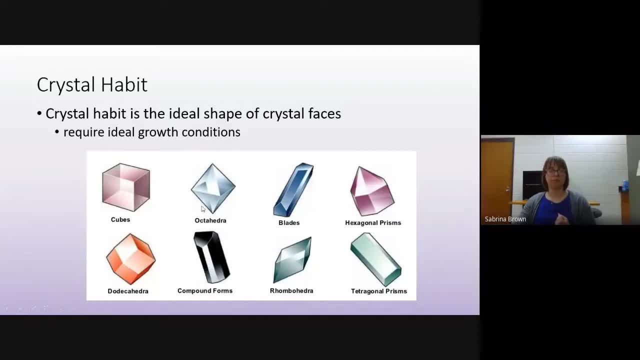 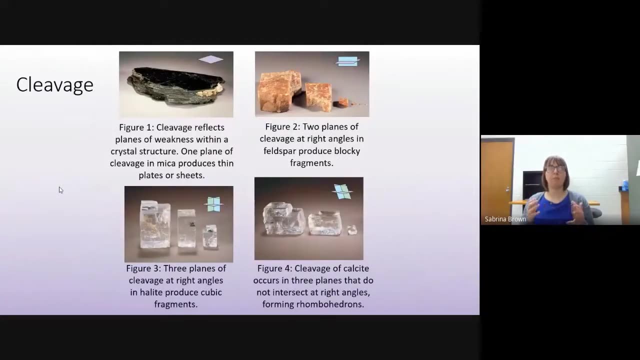 so those are kind of the basic ones we usually cover in this class, Right? so what does the crystal look like if it has an ideal shape? All right. next is cleavage, which is basically the number of planes of weakness within a mineral. So cleavage, it's just telling you that, because of the way that the bonds are, 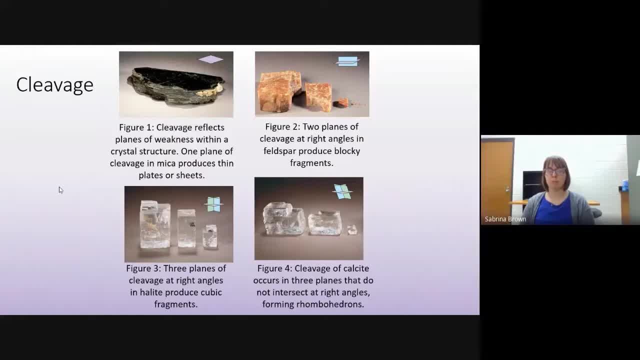 held together. sometimes there are places in the mineral that are more easy to break than others, and if they do not break, then they are definitely not. cleavage break really smoothly in a nice straight line, then that's a plane of weakness, And so that's. 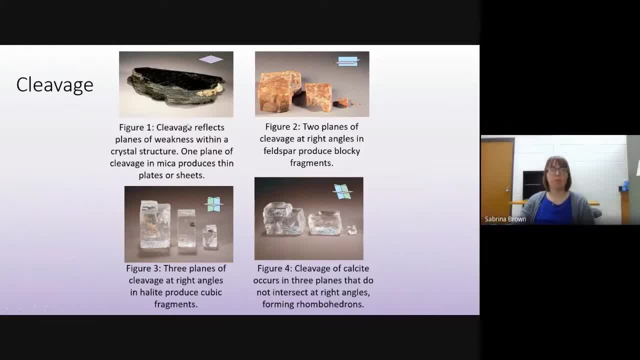 what we call cleavage, these planes of weakness. And when we have one plane of weakness, that means you kind of have this sheet-like shaped mineral. When you have two planes of cleavage at right angles, you kind of have a top and a side and then the other side is broken. When you have three, 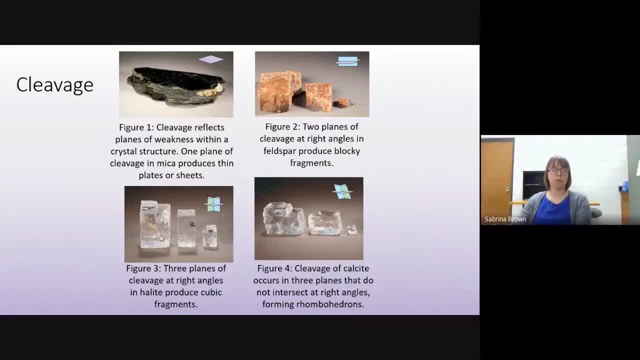 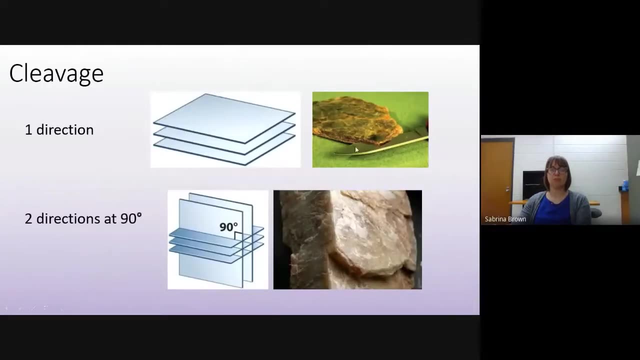 planes of cleavage. at 90 degrees, you get square, rectangular-shaped guys. When you have three planes not at right angles, you get rhombohedral-shaped guys. So here's just more examples of what one direction of cleavage looks like. sorry, two directions at 90. 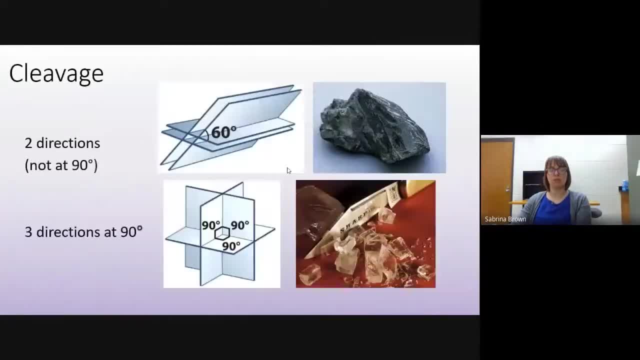 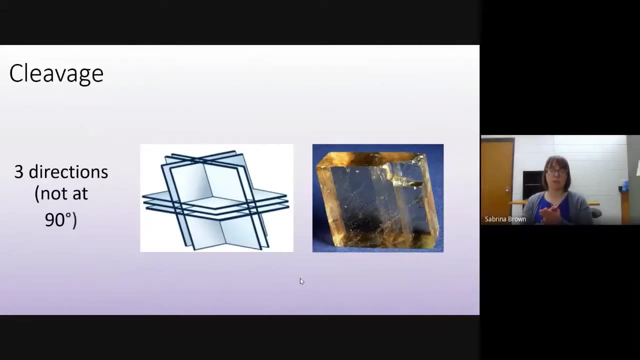 degrees, Two directions at not 90 degrees, three directions at 90 degrees and then three directions at not 90 degrees, And so cleavage is always really challenging, and so when we have our face-to-face class, I promise that I will explain cleavage to you again. 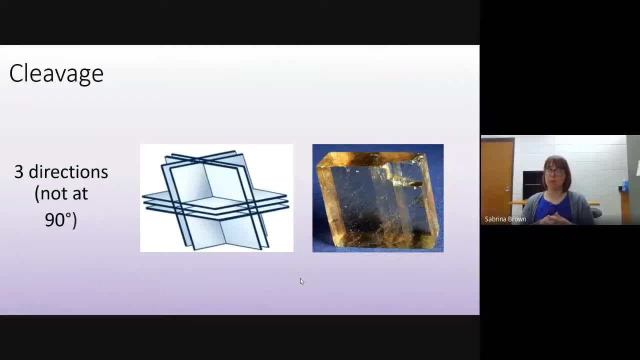 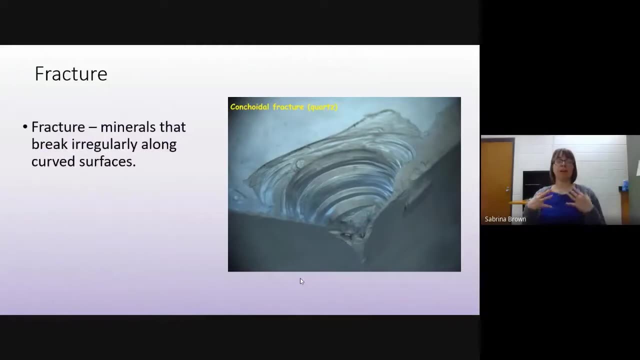 because it's really challenging when we work with the hand samples. we will practice identifying cleavage and identifying those planes of weakness. Some minerals don't have cleavage at all, and so if they have no planes of weakness, then they have what's called fracture, And so fracture is just when minerals break irregularly. 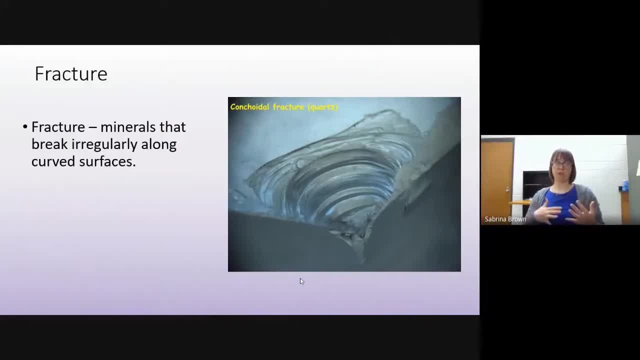 along curved surfaces right. So cleavage and fracture are related. Cleavage is when you have a plane of weakness, Fracture is when you don't have any planes of weakness. And when you have fracture you get sort of this curved shape. If you've ever broken glass. 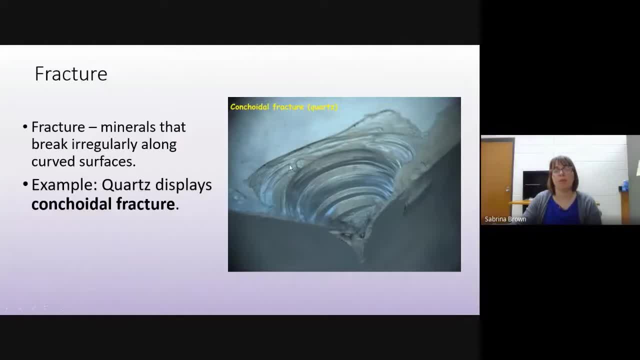 it breaks like this as well, And that's something called conchoidal fracture, right? So conchoidal fracture is one reason why arrowheads are made out of chert and obsidian, because both of those have this conchoidal fracture. It can get fractured. So if you have a plane of weakness, 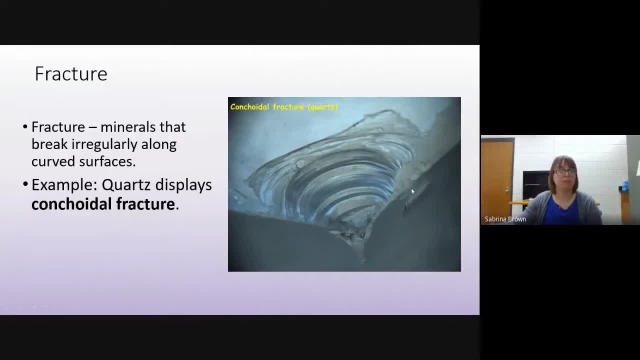 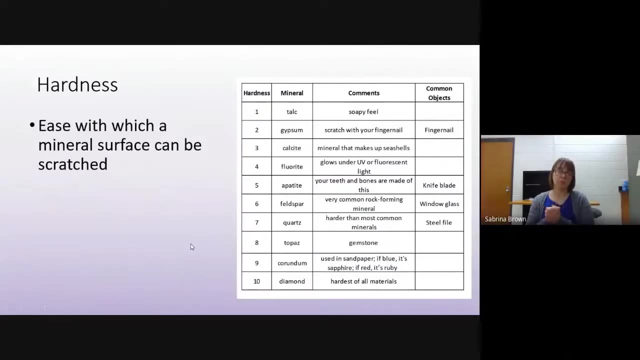 it can get really sharp if you break it the right way. That's why glass gets really sharp when it breaks right, Because of this fracture and resulting conchoidal pattern. All right, so hardness is another physical property that we use to identify minerals. 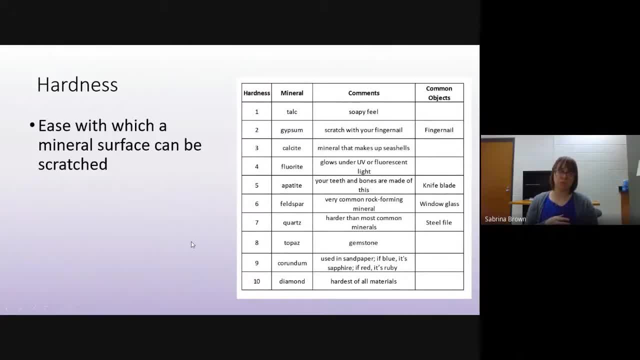 And hardness is just how easy it is to scratch the mineral surface And hardness is related back to how strong those chemical bonds within the mineral are. And what we do in the lab and in the field is use something called the Mohs hardness scale or the Mohs scale of hardness to identify the hardness. 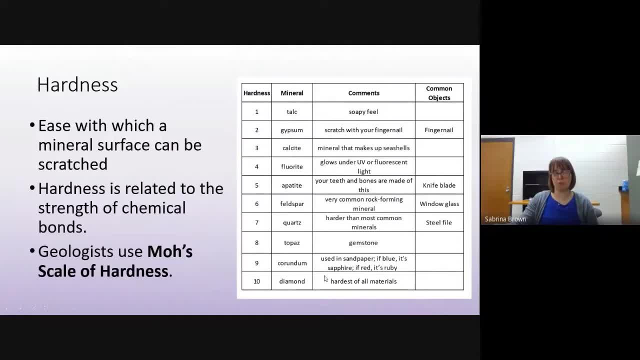 of a mineral, And so the way that you read this table over here- this is the Mohs hardness scale- is that you can see the hardness listed down. here On the left-hand side there's some mineral examples And then some comments about just how cool those are, And then 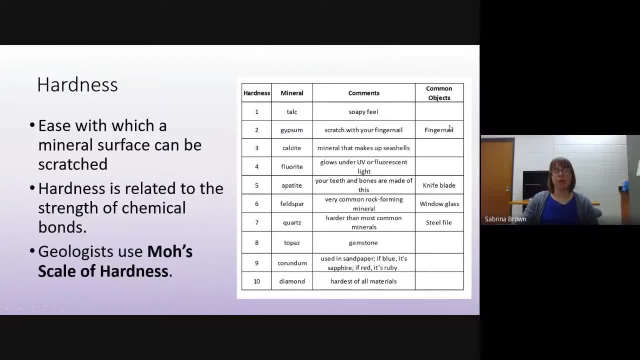 you relate it to common objects. So in the lab we will have a nail, glass steel. Usually we don't have a knife blade. Usually we use nails instead, because they're a similar hardness. But the way that you read this is that the object over here, this is the Mohs hardness scale, And so you can. 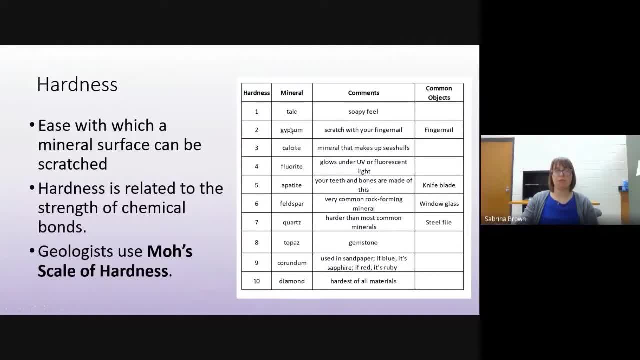 see that this object over here is harder than the mineral that it's in the same line of. So if I asked you which mineral scratches window glass but cannot scratch a steel file, you would say quartz, because quartz is harder than this object- window glass. And so you can see that this object over here 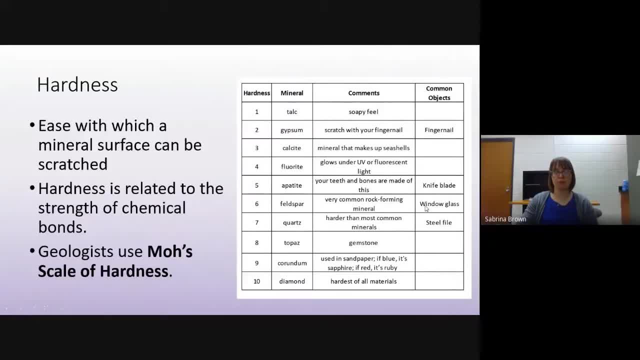 is harder than this glass, And so if you scratched quartz against glass, it would scratch the glass. And if you tried to scratch a steel file with that quartz sample, what would happen is that the steel file will actually scratch quartz. And so, again, we will practice this in the lab. It's 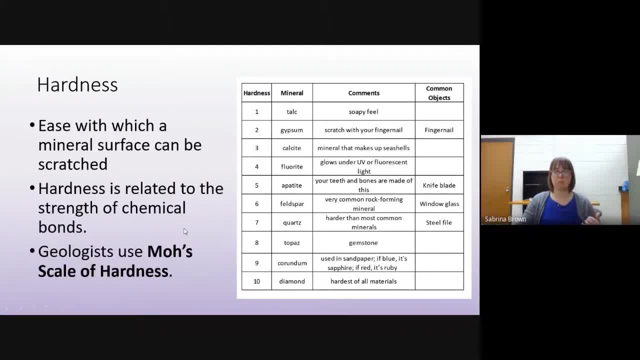 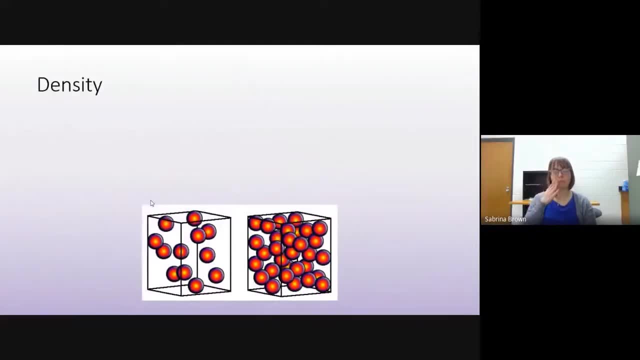 okay, if you don't understand it right now, We will get lots of practice with reading the Mohs hardness scale and identifying hardness. The�도 is another physical property that's used to identify minerals. is basically the ratio of the weight of a substance to its volume. Again, that depends on the elements that make up the mineral. 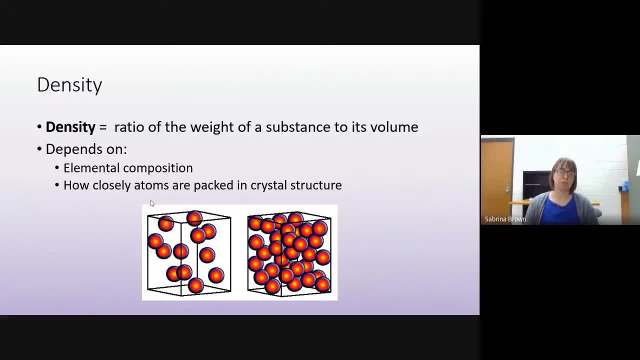 and how closely the atoms are packed together within that crystal structure. We don't sort of actively use density or measure it in the lab, but what we? but, um, you know, we use density if you you pick up a sample and you're like wow, that's really light or wow, that's really heavy. 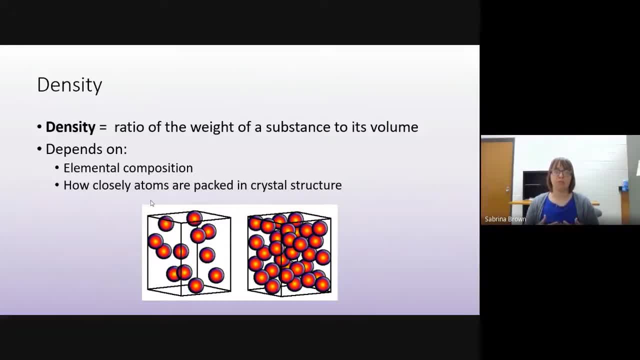 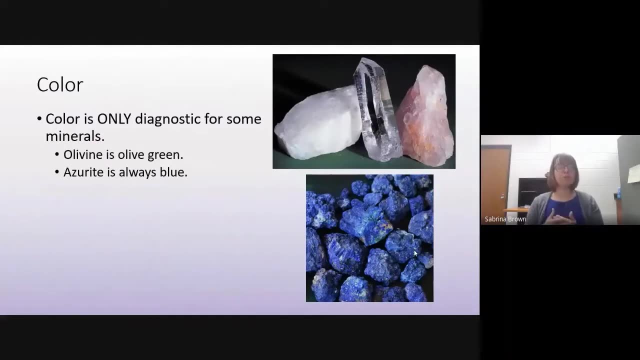 in weight, then that has to do with density, and so we sort of we don't really do anything official with it in lab, but it is something that you sense just by picking up the mineral samples. so color is the next diagnostic property, and it's a little weird because it's only diagnostic. 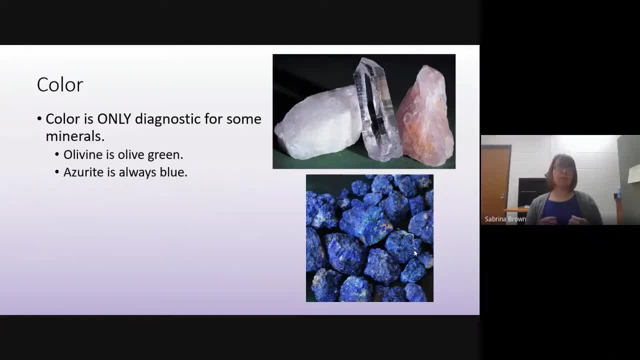 for some minerals, and what that means is that some minerals are always a certain color. so, for example, the mineral olivine is always olive green colored, or the mineral azurite is always blue colored, but for the most part, a lot of minerals can be a range of colors. 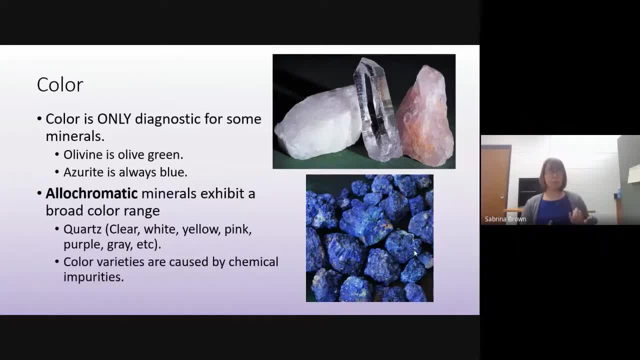 and so we call those minerals that are more than one color alichromatic, and so, for example, alichromatic minerals, uh, an example would be quartz. so quartz can be clear, it can be white, it can be yellow, pink, purple, gray, black, it can be all kinds of colors. so here's an example of three. 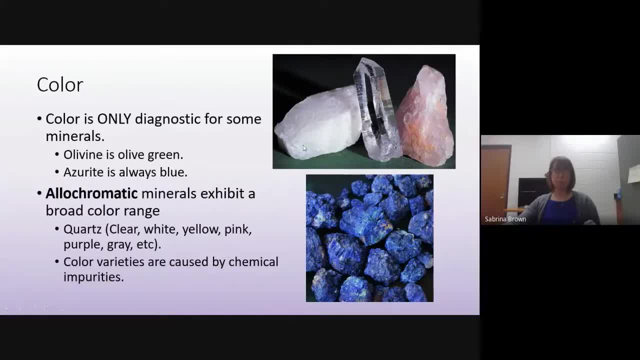 different types of quartz up here, and minerals are alichromatic. minerals are different colors because there are chemical impurities within them which create these slightly different colors, and so when you're using color in the lab to identify minerals, be very careful, using color as like the top diagnostic property. 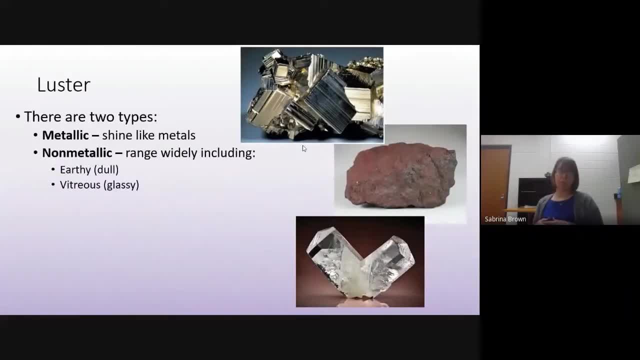 another physical property that we can use to identify minerals is something called luster, and there are two main types of luster. the first is metallic, which means that the mineral is shiny like a metal- like this pyrite up here is shiny like a metal. and then the other type is non-metallic. 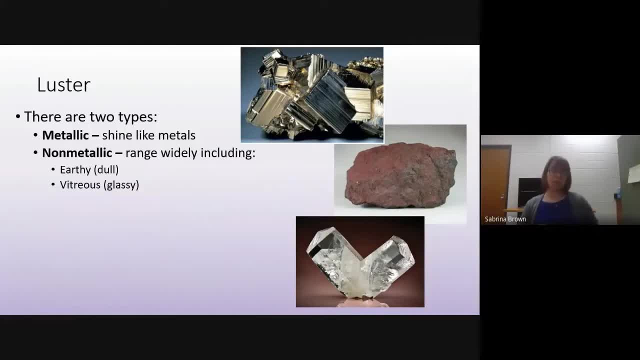 and non-metallic just means that it's not shiny like a metal. it can be sort of reflective like a glass, like this quartz down here, so don't get confused when you're thinking: well, metal is shiny, so anything that's sort of reflecting light is metallic. 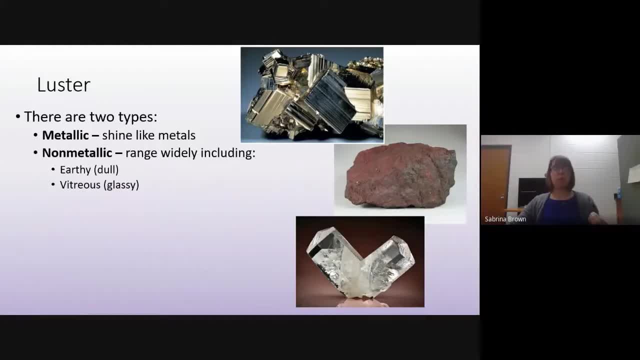 metallic is just things that look like metal. non-metallic is everything else, which include vitreous or glassy things like quartz, and even dull minerals or earthy minerals that have no shine at all. we can also describe minerals as transparent, which means that you can see through the mineral. 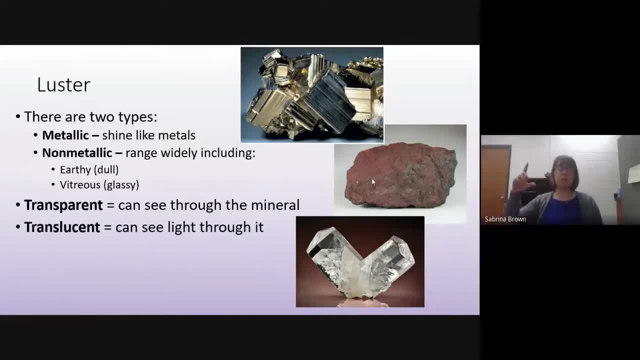 translucent, which means that if you hold it up to the light, you can see light through it, but you can't see through it. i always say the different difference between transparent and translucent is that if you put a transparent mineral down on a piece of paper, you could read through it. 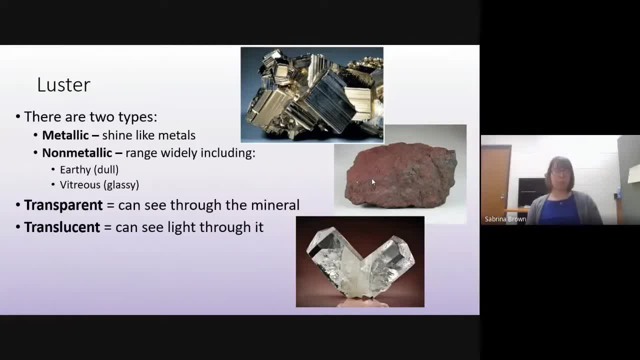 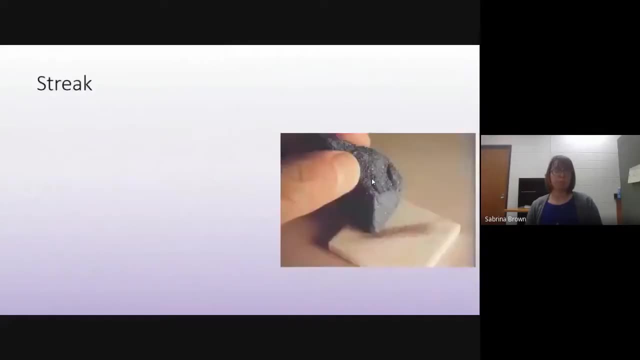 if you put a translucent mineral down on a piece of paper, you could see the white through it, but you couldn't read the words on the other side. and then we have opaque minerals which you can't see through or into at all. so you can crisscross and see the white through the white and then you can see that the white goes. 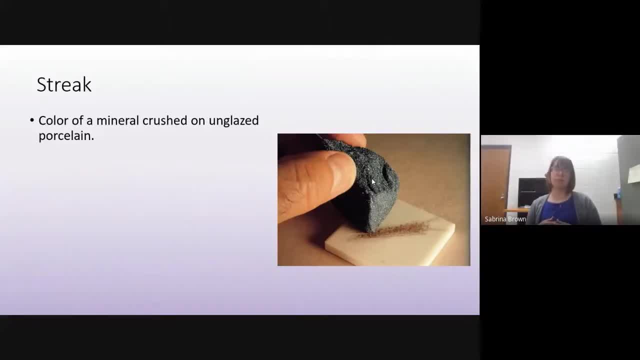 however, we can say that the white is transparent, because when we see the grey it's transparent. so now let's also look at the physical properties of streaks. finally, the physical property: streak is the color of a mineral when it is crushed onto a piece of unglazed porcelain. so we call it streak because you streak it across this piece of porcelain. 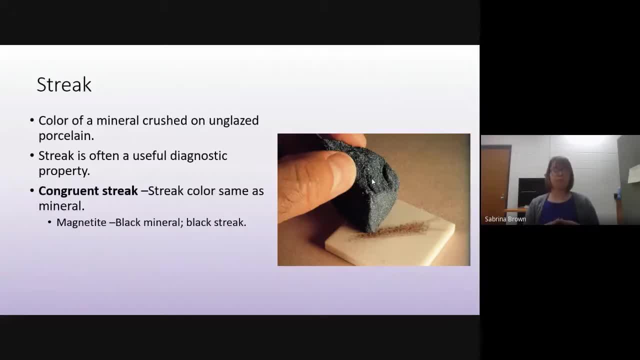 have congruent streak and that just means that the streak color is the same color as the mineral. So, for example, magnetite is a black mineral and when you streak it across an unglazed porcelain plate it leaves a black streak behind. But there's also something called incongruent streak. 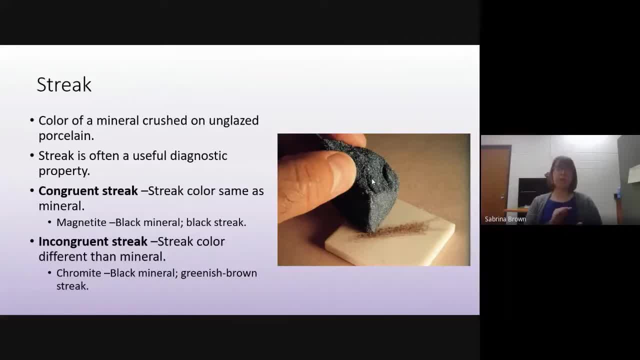 which is when you streak the mineral and the streak is a different color than the mineral itself. So, for example, chromite is black, but when you streak it it has this greenish-brown color, And so you can tell the difference between magnetite and chromite in the lab. 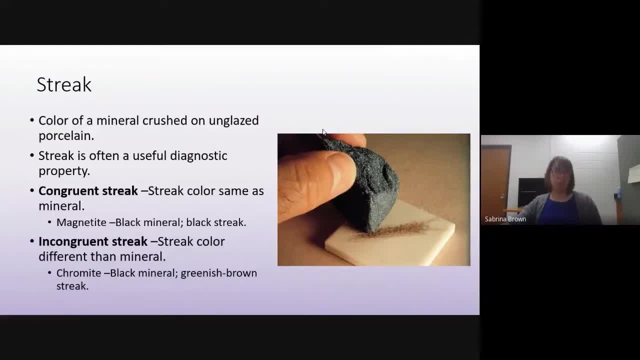 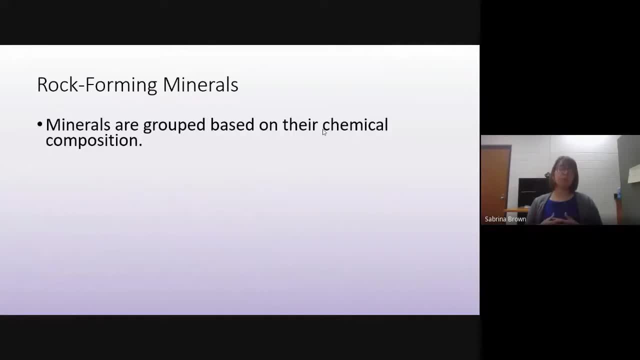 by streak, even though they look the same when you just hold them in your hand. All right, and so minerals. we group them together based on their chemical composition, And we'll get more into chemical composition in a little bit. We'll get more into chemical composition as we move on in the class and we'll talk about 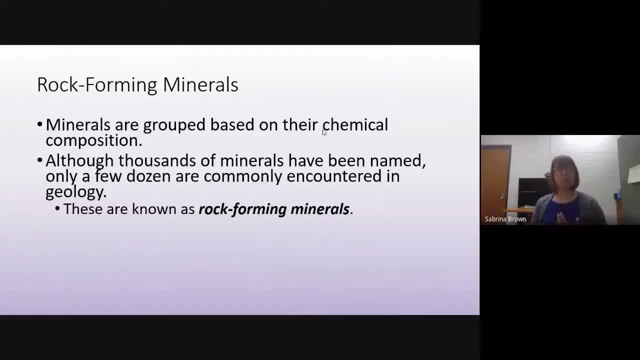 silicate minerals and non-silicate minerals, But just for now, know that we largely group minerals based on what chemicals they're made up of, And even though there's thousands of minerals that have names, we only end up talking about a few dozen of them in environmental science. 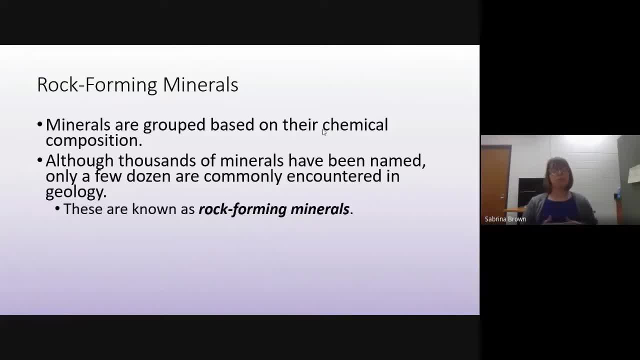 class, And that's because there's only a few dozen that are commonly encountered on Earth. And we call those minerals and we call them minerals, and we call them minerals and we call those minerals rock-forming minerals because they make up the majority of rocks on Earth. 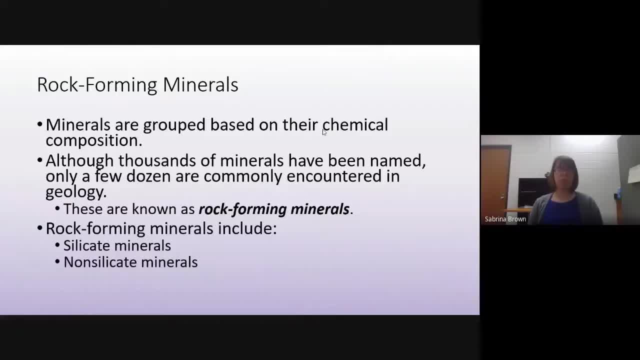 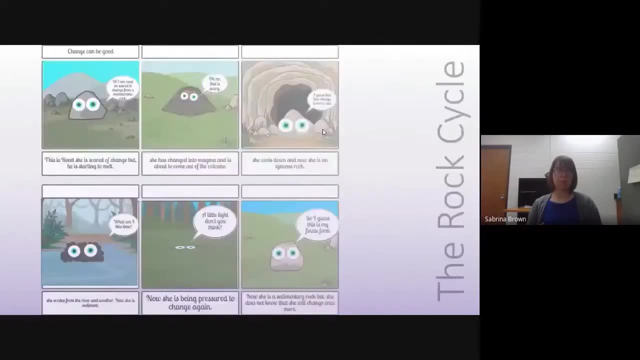 And those rock-forming minerals, as I mentioned, include silicate and non-silicate minerals, which we will talk about as we start to talk about rocks, volcanoes, et cetera. All right, and so let's talk briefly about the rock cycle. 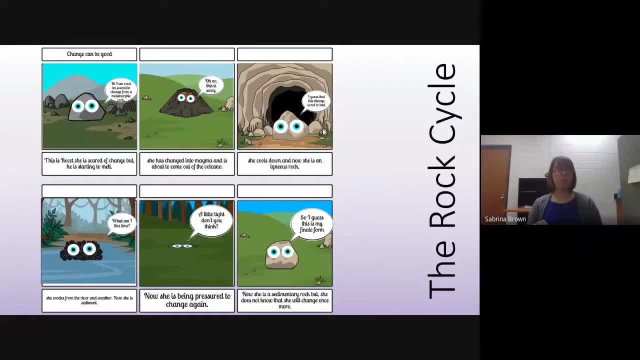 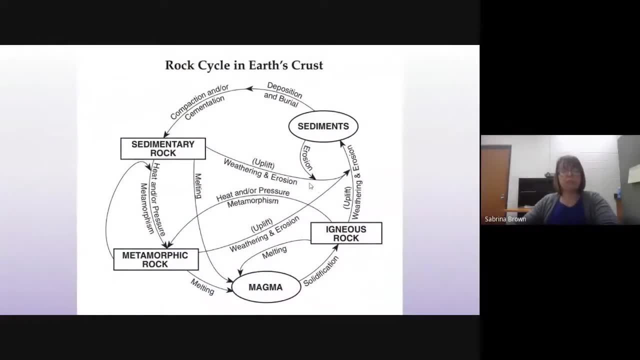 And then in class we will do some more with the rock cycle. And so remember, there are three types of rocks: We have igneous rocks, we have sedimentary rocks and we have metamorphic rocks. So think back. You learned this once in your life, I know. 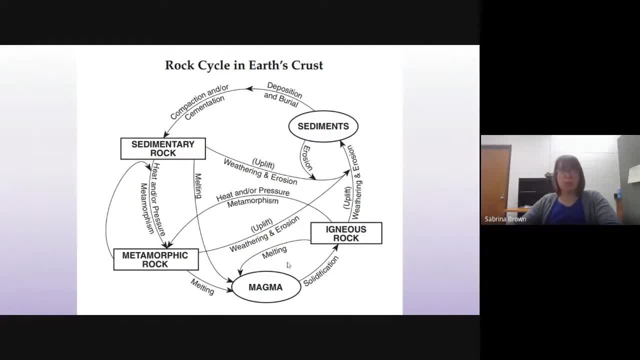 Might have been in elementary school, but you learned it, I'm sure. So let's start down here with magma on the rock cycle, And we're going to talk about magma on the rock cycle, And we're going to talk about magma on the rock cycle, And so we have magma which is molten rock, And if we cool and 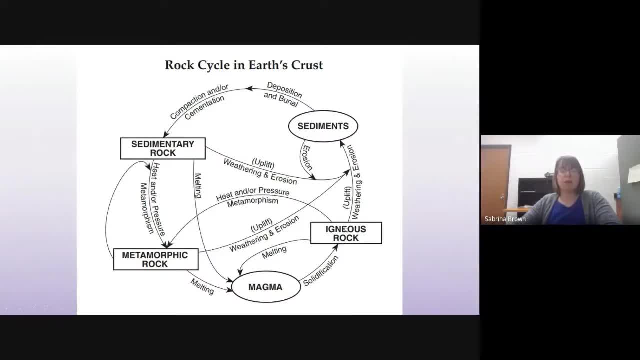 solidify magma, we get an igneous rock, because igneous rocks are formed from the cooling and solidification of magma or lava. So then our igneous rock can turn into a couple of different things. One: it can melt back into magma. 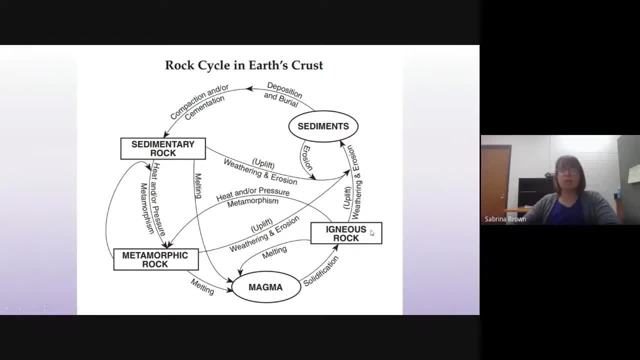 So our igneous rock can melt and turn into magma. Our igneous rock can also be weathered and eroded, so broken up into little pieces, which we call sediments. And our igneous rock can also undergo heat and pressure through the process we call metamorphism, and turn into a metamorphic rock. 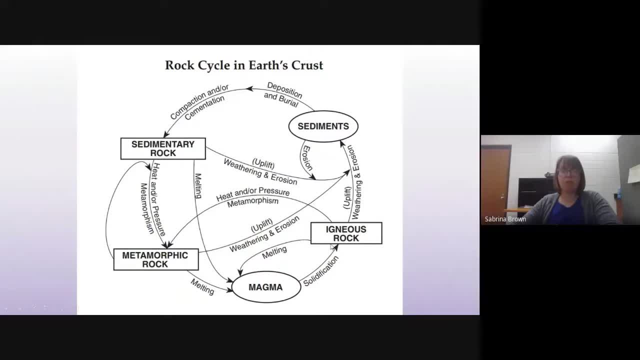 So again, our igneous rock can melt and turn into magma, And our igneous rock can also be weathered and eroded. which formed from magma can either turn back into magma, it can be weathered and eroded in sediments. 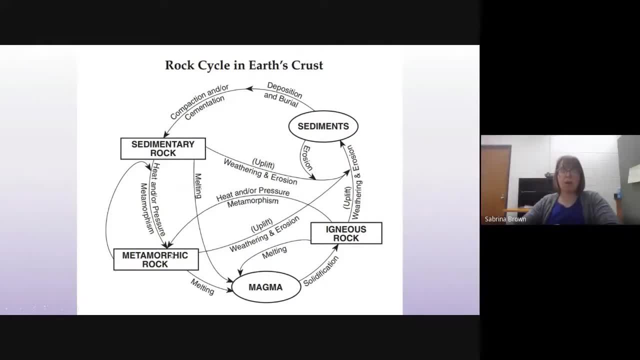 or it can undergo heat and pressure and turn into a metamorphic rock. So we always say about the rock cycle: rocks can turn into any other type of rock or into themselves again. So, for example, our igneous rock can melt into magma, which then solidifies.